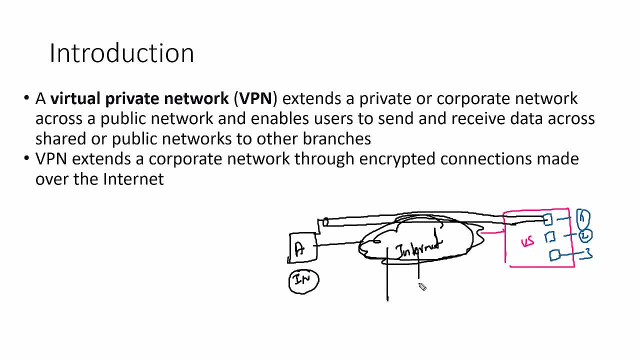 he's sending a request on the internet directly. there is a possibility that we have a multiple attackers. okay, there are some multiple attackers: attacker one, attacker to attacker three. so they will try to intercept the data. so, VPN providing them opportunity to create a secure tunnel. okay, it creating a secure. 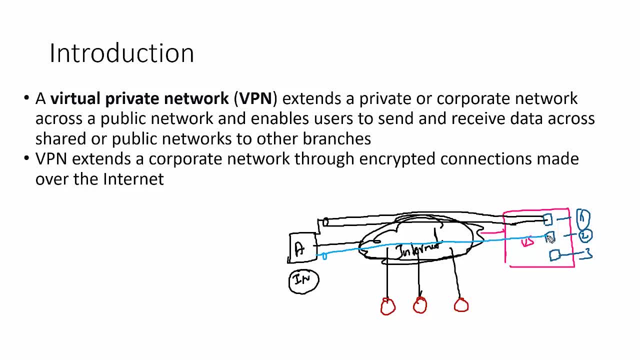 eternal, and then, through this particular tunnel, we basically send the data. so a just feel like that he is a part of an enterprise and by this he can able to access the resource one, resource two and resource three- same. like we have a other branch, so this is the branch. instead of a system, we have a branch. 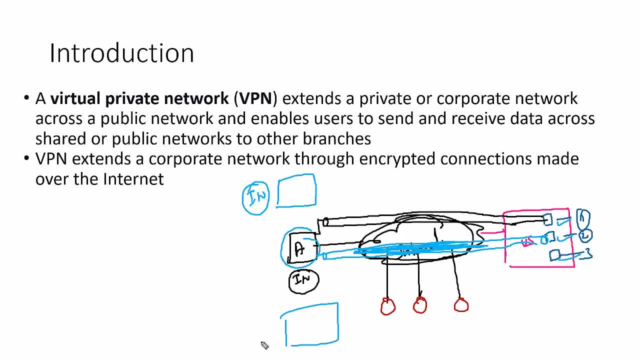 branch in India and branch in UK, head office in us. okay, so now what happened? with the help of VPN, my internal user can able to access other location resources. my internal user, with the help of Internet, can able to access the other branches resources. so, by this way, this private network was extended, with the help of VPN, over the public to 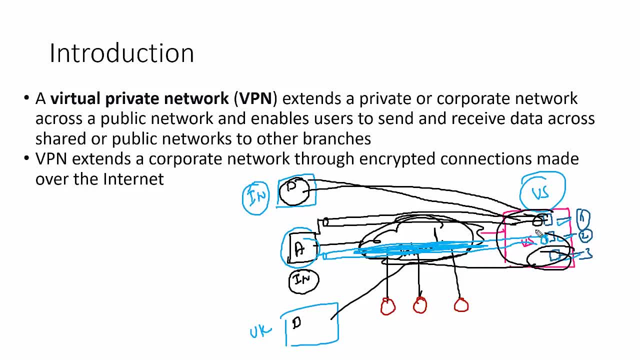 connect with the branch. so this is what is VPN. so VPN extend a private corporate network, private or corporate network across the public network. enable the user to send and receive data across a shared or public network to the other branch. One more example: like in India, we have a metros. In US also, we have a private train. So it was created over the. 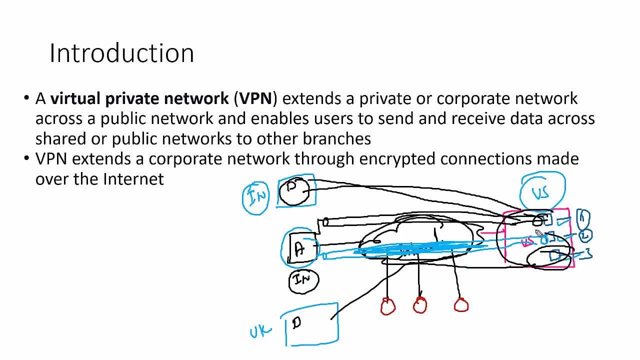 public traffic And if you go by the train, we can able to reach from one location to the location as early as possible Because they have a separate route, They have a separate channel by which it basically travel And that basically save our time, Same like we have a VPN. 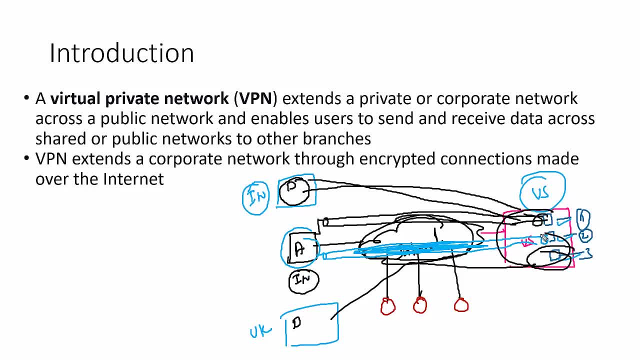 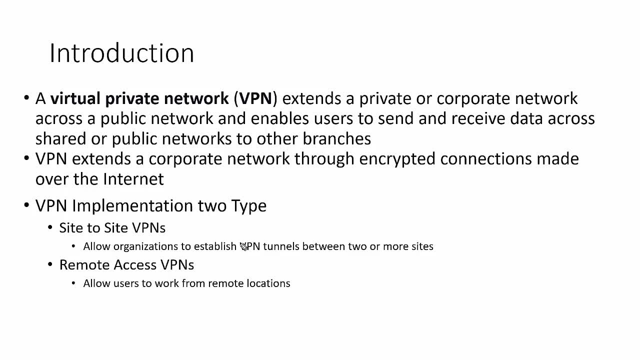 which was introduced initially with this purpose. So when we are talking about the VPN implementation, VPN is basically implement by two way. One is called as a site to site VPN and second is called as a remote access VPN. As I said, we have a branch office in India. 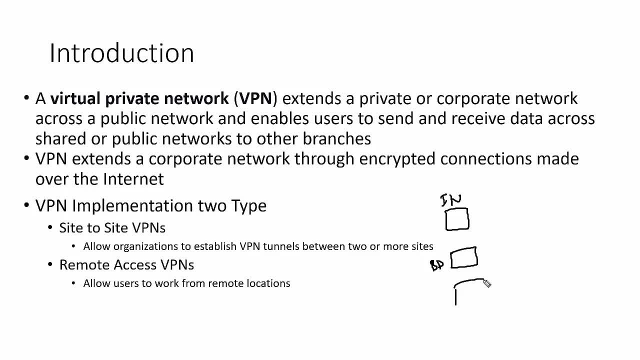 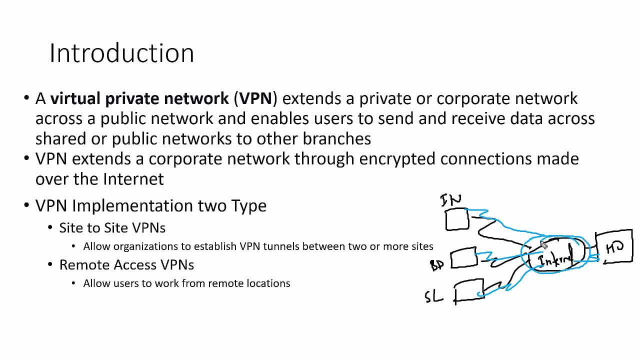 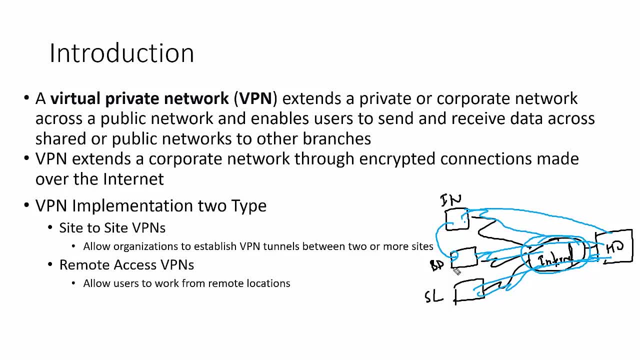 So that is what is called as a site to site VPN. So that is what is called as a site to site VPN. But if there is a one user from his home trying to connect only with that office using a VPN, connect with the head office. that is part of the remote access VPN. 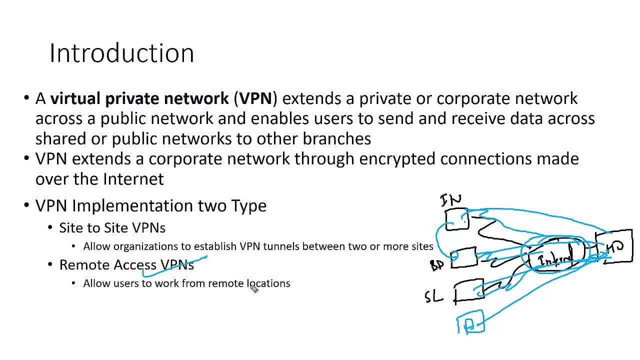 Simple, like I am at home and I am connecting with my branch office, I am connecting with my enterprise, So that is a remote access VPN, or we have a multiple branches. They are sharing a data on a regular basis. With the help of VPN, they can able to build a network seamlessly. They can able to communicate across the network. 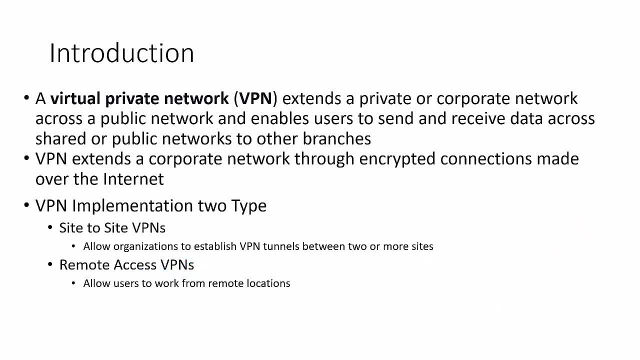 So that is basically called as a site to site VPN. So that is basically called as a site to site VPN. Now, in a layman, I can explain you how the VPN works. So we have a system, A- Okay, and this is my head office. 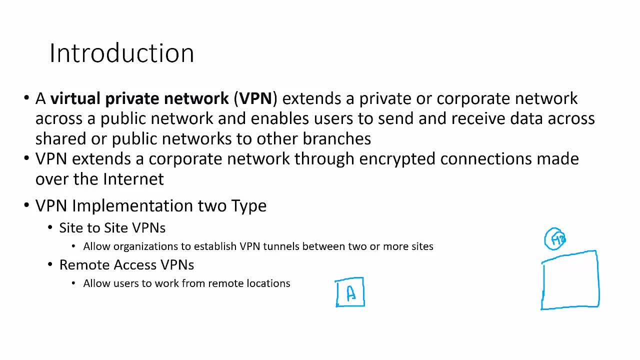 So we have a VPN server here. imagine- Let me draw it more effectively- So we have a user system A And this is basically my branch office. Okay, So we have a VPN server here. okay, so we have a VPN server now. user is basically first dial the IP. they. 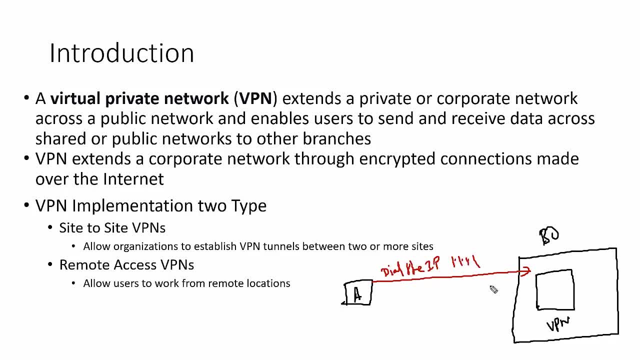 dial the IP. example: one dot one, dot, one dot one. this request is basically carry on the PPP. you know why? because the devices which is configured on the internet, they are the DT DC devices. DT DC devices, they don't understand the IP packet. and all that so that the dial-up request is carried by the PPP protocol. 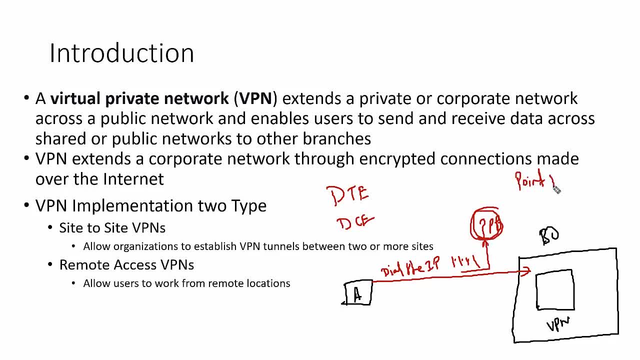 which is called as a point-to-point protocol. so the DT DC device can able to understand and by this way they able to pass the information to VPN server. the VPN server is basically asked for the username and password. so this kind of a pop-up we get: enter the username and enter the password. so 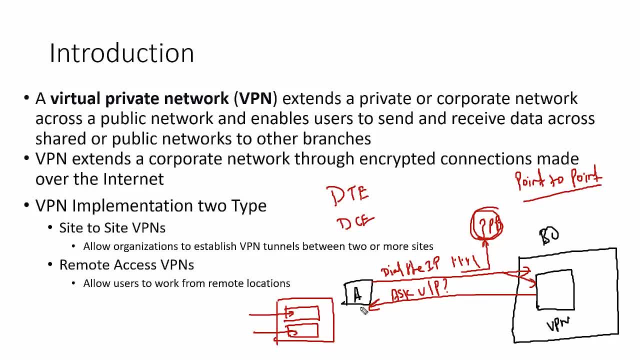 there's a username and password we basically enter. when we enter the username password, default. here we use mostly chap authentication. okay, that's why you can see some kind of a blue pop-up when you connect with any server which ask for the credential called as a username and password. so we enter. 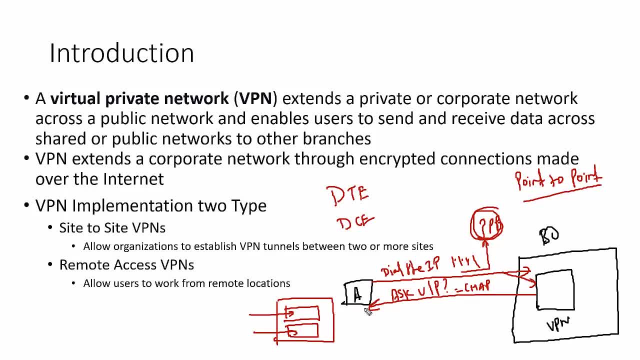 username, we enter the password. when we enter the username password, that information sent to VPN and then we basically create a channel. this is the tunnel has been created. so, over the when, this is the tunnel we created and through this particular tunnel we transfer the data- now your tunnel creating between the user- to the location. then it is a remote. 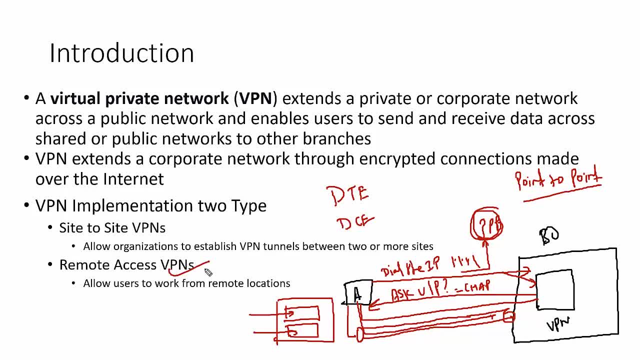 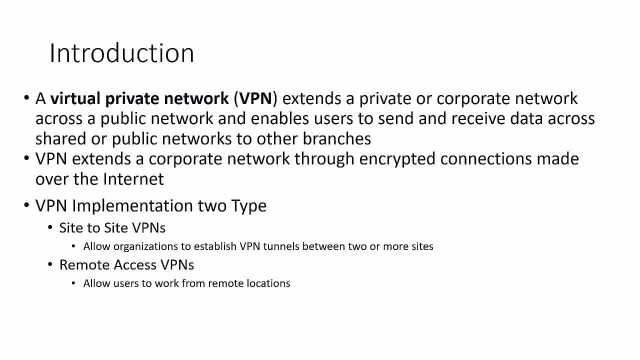 access VPN, the tunnel created between the two branch that is called as a site-to-site VPN. okay, so this is how the VPN basically works. so it establish the secure channel over the internet by we lake a able to send the date have without any issues in everything and by this way. 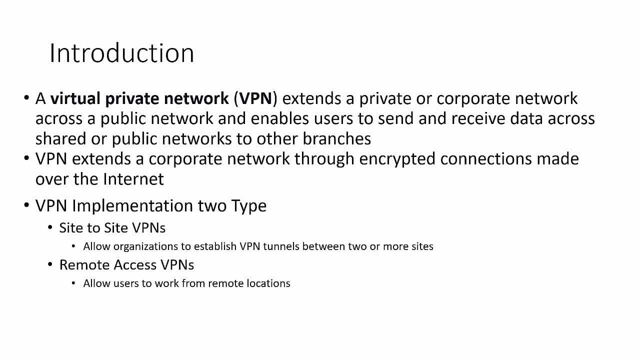 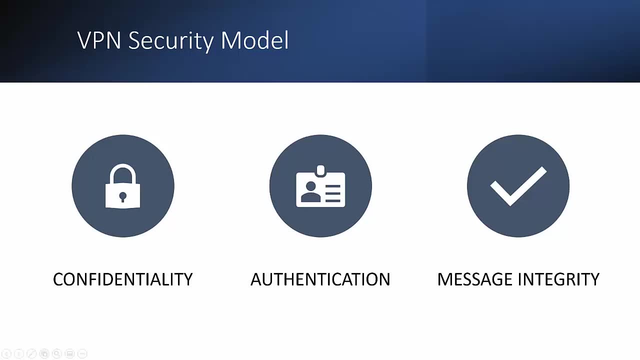 we have a sending of the data. so now we're going to discuss about the different type of tunnel, but before that in VPN, we also need to understand the security model. so when we going for the VPN, it offer three important things. first, is called as a confidentiality, so confidentiality mean it creating a separate tunnel through. 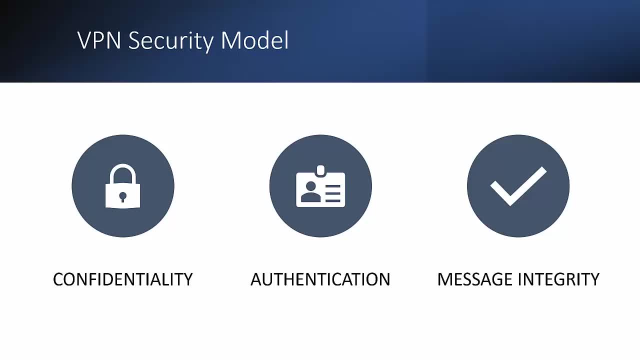 which it send the data, so it can protect against sniffing and all that. so that is the best thing about VPN. second, is it offered the authentication which prevent unauthorized user from accessing the VPN? definitely, when you're connecting with any branch office and all that, it need a username and password until then, as you. 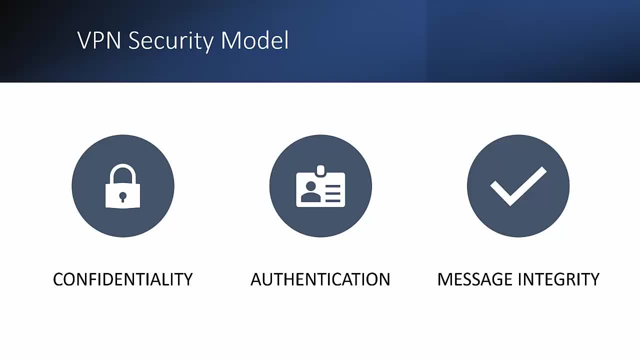 don't have a username password, you can't able to connect with them. so by this way we ensure only the authorized users to be part of or connect to the branch office. they also use the hashing and all that by which they ensure that okay message should not be altered. that is, a VPN is rely on the external solution. 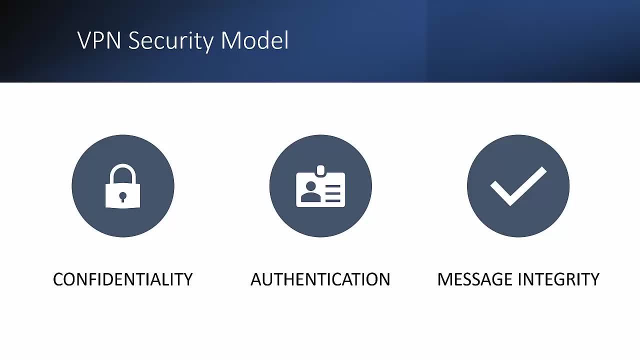 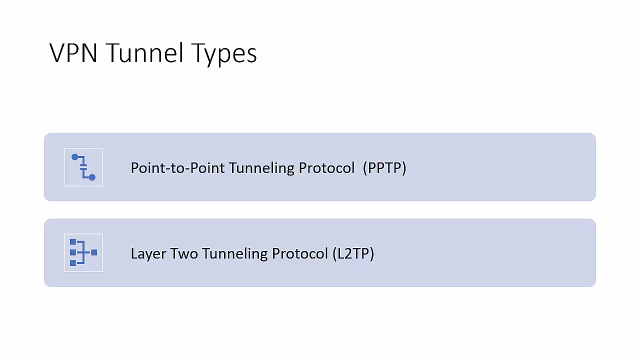 which is called as IPSec. okay, okay, so these are three important security models are used in a VPN, okay. protection against unauthorized disclosure: okay, make sure only authorized user can able to connect. and third, protect against the unauthorized modification. now we're going to discuss about the VPN tunnel, okay, so next part is VPN tunnel types. we 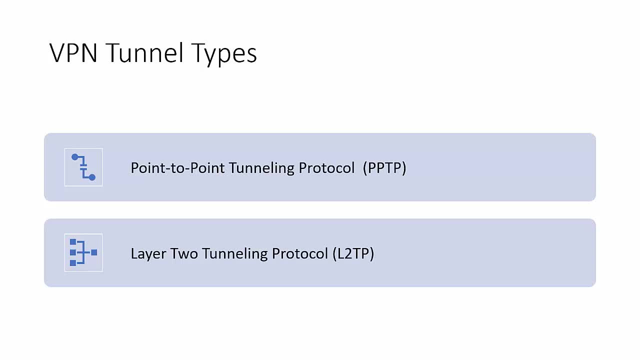 have a two type of tunnels: PPTP and L2TP. we also have a third which is called SSL VPN, and all that as we're covering more from an interview and exam preparation, so I thought I will limit it to two only because these are the base. so in this, 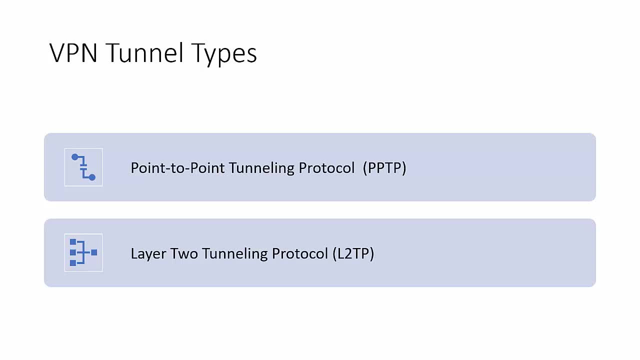 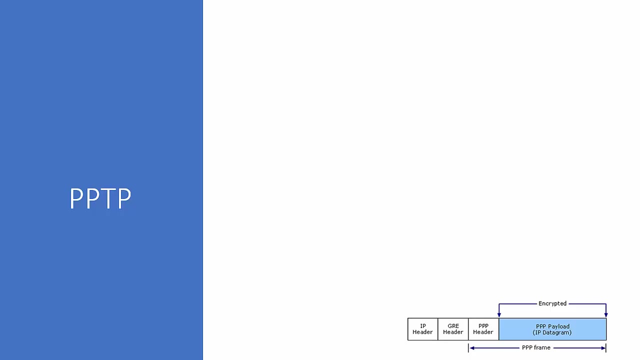 section we're going to discuss a PPTP, L2TP, because when you're talking about tunnel, tunnel we create in the site to site and tunnel we create in the remote user. so the first part: we're going to discuss about PPTP. okay, so first we're going to discuss about PPTP. if you go by the description, 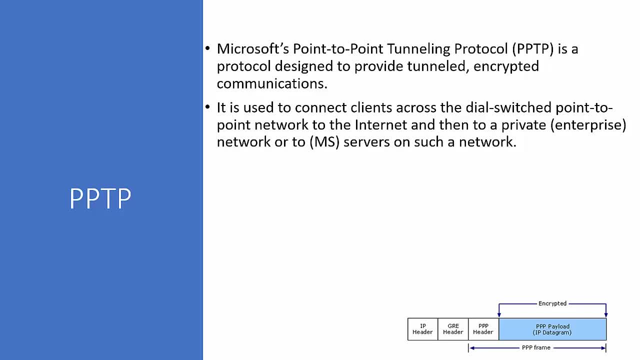 of PPTP. it's saying it's Microsoft point-to-point tunneling protocol. you are absolutely right. it is basically developed by Microsoft, so that's why it is called as a Microsoft point-to-point tunneling protocol, which is designed to provide tunnel tunnel in scripted communication. ok, so it is used to connect client. 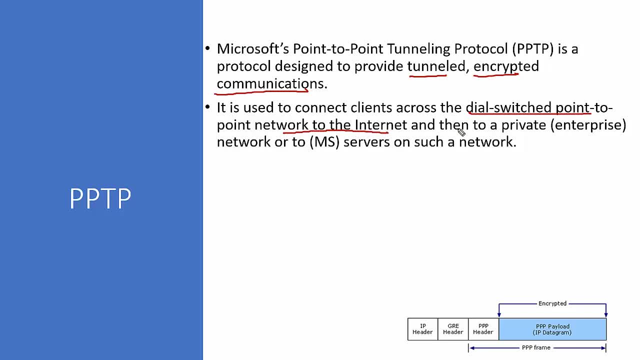 across the dial, switch point-to-point Network to the Internet and then to the private enterprise network, to the ems servers on such networks. if we're talking about the package structure of the PPTB, before going to discuss about a package structure, let me explain in the process. so we have a user here connected with the internet. 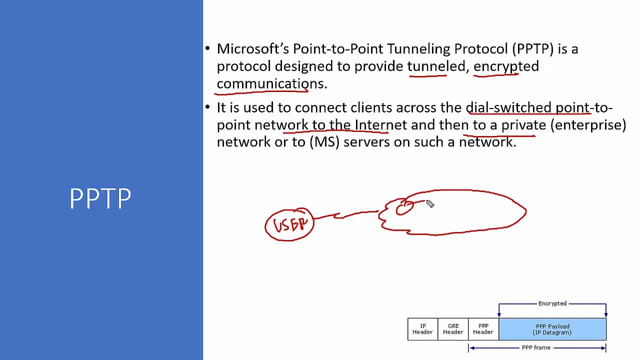 so we have a router, one router to router three. so we have our routers here and here we have a VPN server. this is the Microsoft RAS server, you can say. and then from there we connected with the system a, system B, system C. so this is basically my enterprise, you can see like that. 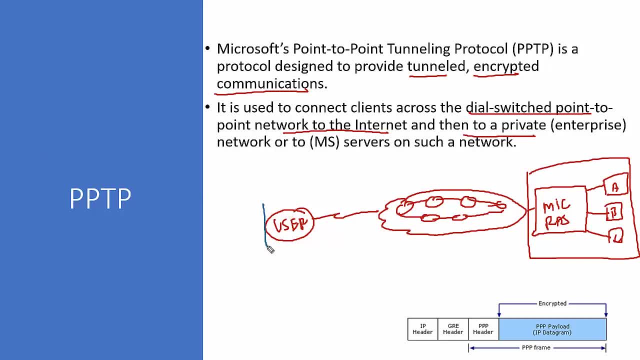 okay, so user wish to be connect with the enterprise network so you can able to access the resources. so user does the dial-up. definitely, when you're doing dial-up, these protocols only understand layer 2, so by this the information carry to the Microsoft RAS server. now, when this carry, this is basically. 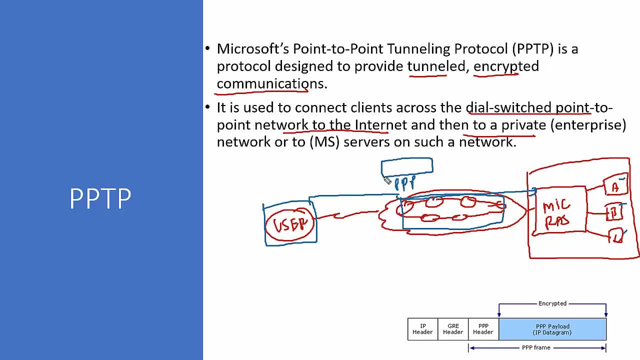 carry by the PPP. on top of it we also add the PPTP protocol, because Microsoft will not able to understand the layer 2 communication. we need something like a layer 3 communication protocol. so Microsoft will not able to understand PPP. so we basically carry PPTP request with PPP then. 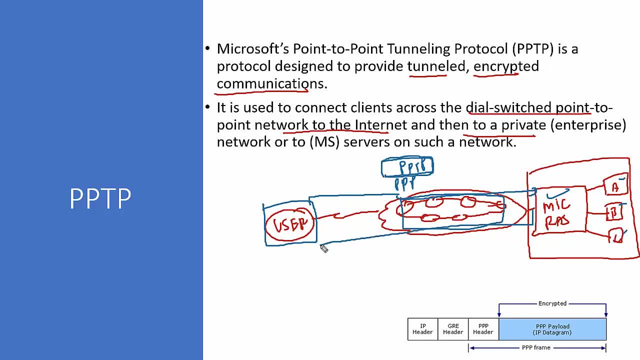 Microsoft. when it received the request, it basically asked for the user name and password. Microsoft is using a pap and chap. primarily it used chap, which is called as a challenge handle handshake authentication protocol, where the Microsoft will send the nonce value. so when they send the username password it has a nonce value. that's why you know, sometime you notice you get a. 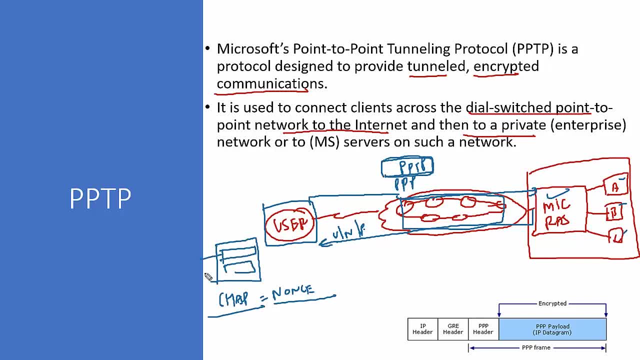 login pop-up so you enter the username, you enter the password. that password is used to encrypt the nonce and it send it back to the Microsoft server. Microsoft basically verify, validate by decrypting with the same key. if we decrypt successfully, there is a tunnel has been created and then, through the 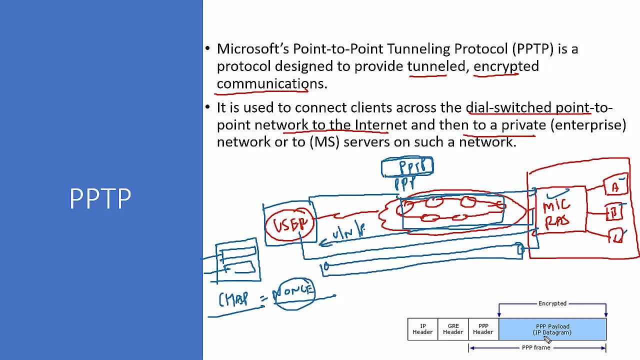 tunnel. we transfer the data and then we send it back to the Microsoft server. so this is basically the packet format. we have any talking about tunnel. so we have a IP datagram, PPP payload, which is purely encrypted. so in PPTP we use one encryption which is called as an MPP- Microsoft point-to-point. 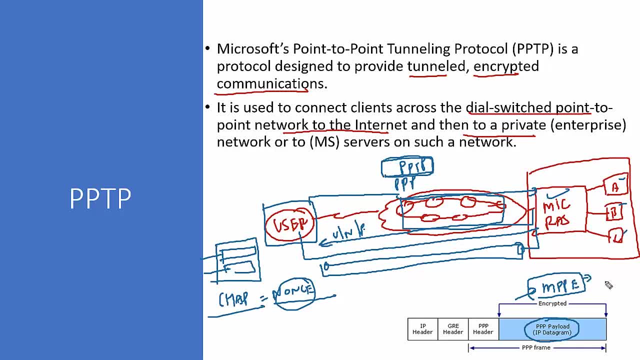 encryption which is used to encrypt this data, and this protocol is used, the RC for algorithm to encrypt the data, which is a symmetric encryption. then we add the PPP header, which is understand by the layer to DT device and DC device. then we have a GRE header and 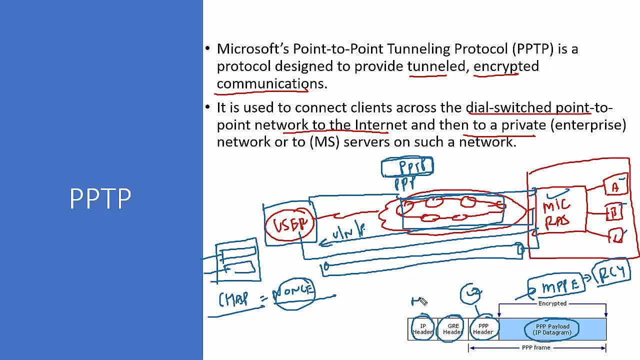 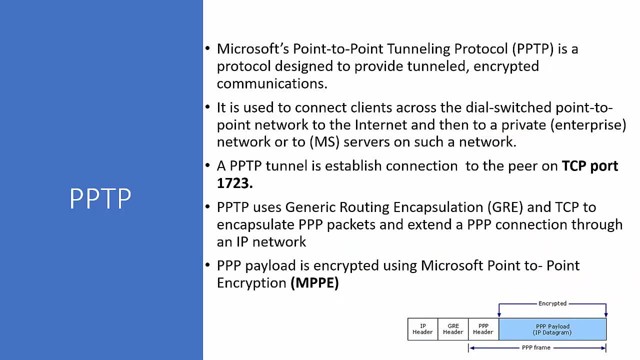 which is for the routing, and then we have IP header for the network layer information. so this is how the PPTP is basically work. so PPTP tunnel established a connection on the TCP port number 1723. most of most cases, the interview will basically ask this question: PPTP use GRE and. 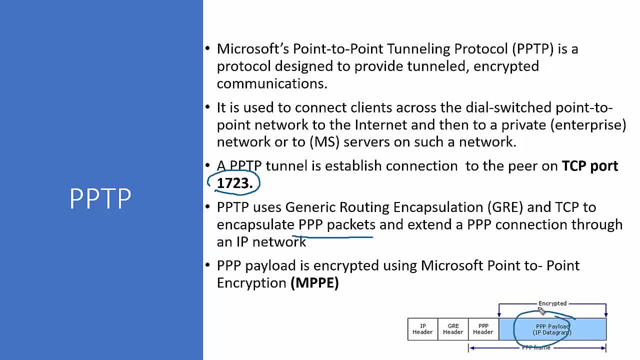 TCP to encapsulate the PV packet. this is what we happen and extend the PP connection to the IP network because IP will not understand the PPTP PPP. so that's why we encapsulate that into PPTP, so that IP network, which is a Microsoft gateways, will understand default PPTP use MPP encryption. 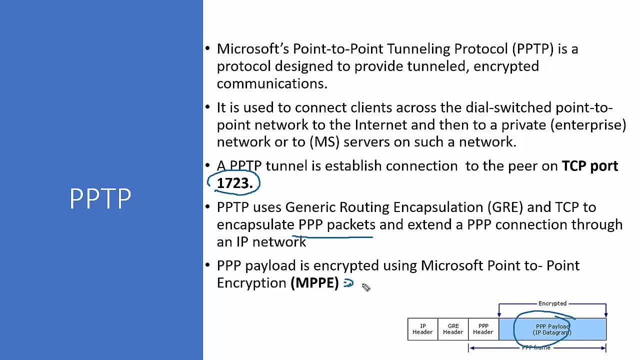 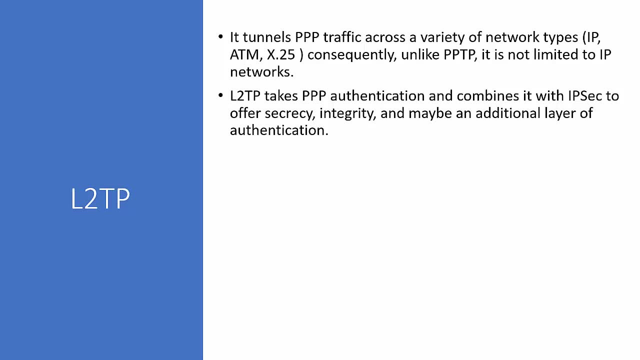 which is called as a Microsoft point-to-point encryption, and MPP use one algorithm, which is called as a RC for. so that is basically all about the PPTP. now let's discuss about the L2 TP. so when you're talking about the L2 TP, L2 TP is a tunnel, which is so Microsoft has some limitation that it. 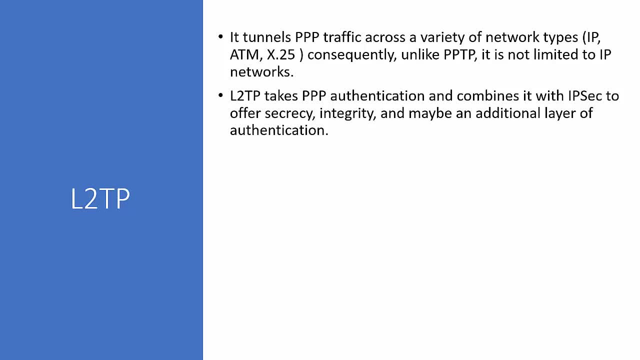 can support above layer 3 communications and everything, layer 3 communications and everything. the internet is configured on x.25, internet is configured on the ATM, internet is configured on the layer 2 communications, layer 2 technologies. and all that because PPTP only work on the. 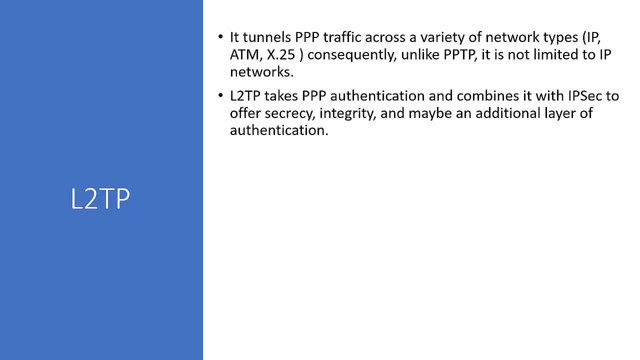 Microsoft IP networks and all that. so we are looking for such solution there. the Cisco come into the picture and Cisco basically introduced the L2 TP layer 2 tunnel protocol. so L2 TP take PPP authentication and combine with IPSec to offer the secrecy, integrity and 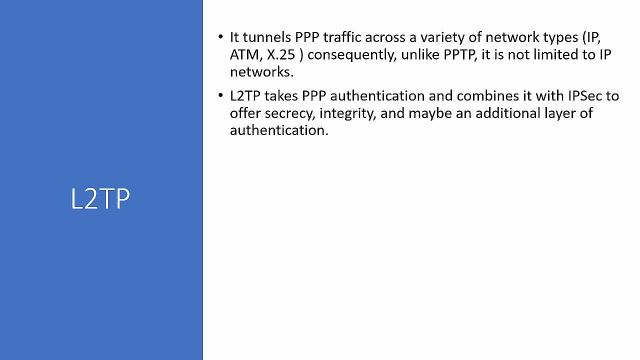 additional layer of authentication. I covered the dedicated IPSec topic in my youtube video. you can check that. so yes, L2 TP default does not have an encryption like the way PPTP- at least have a MPP- L2 TP does not have a default encryption. he has to rely on IPSec for that. so with the help of IPSec, 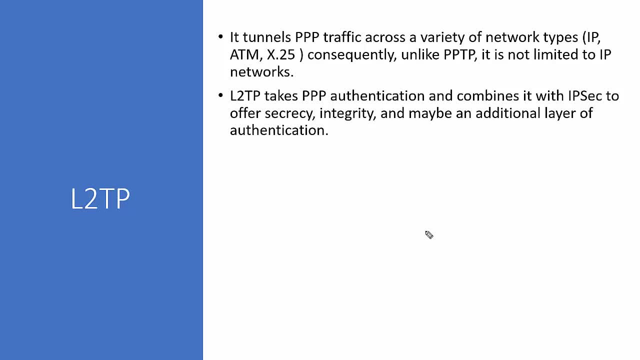 it can offer the you know: confidentiality, authentication and integrity. if you're talking about a high-level IPSec, let me share the mind map of IPSec. so IPSec is the protocol suit to protect the IP packets. so it has a modes, it has a protocol and it has a key management. so when 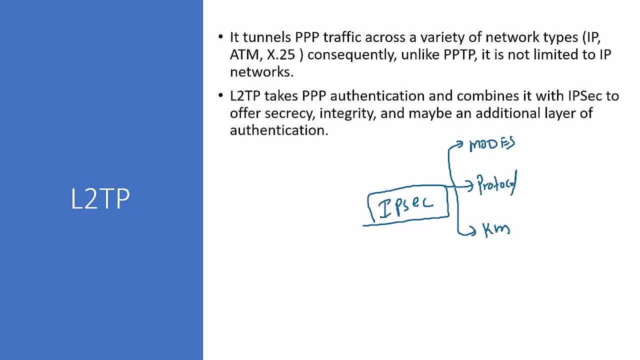 you're talking about the modes. we have a two modes here, so we have a transport mode and we have a tunnel mode. then we have a protocol which is basically called a H and a ESP. first we introduce a H, which offer only authenticity and integrity. later on, ESP was. 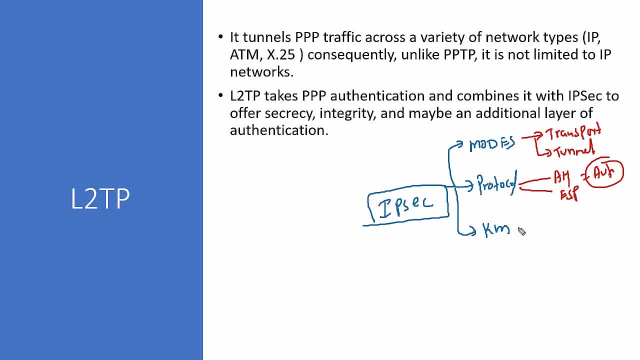 introduced which address both confidentiality, authenticity, integrity. for the key management, we have a IK internet key exchange which basically some of IAC, KMP and Oakley IPSec default use AES for the encryption and for the hashing it use SHA. okay, so that is the function of IPSec for a digital 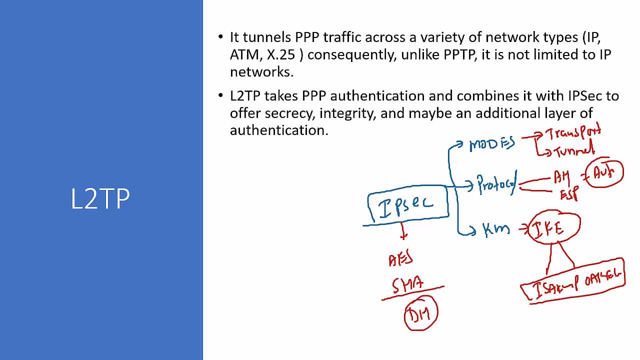 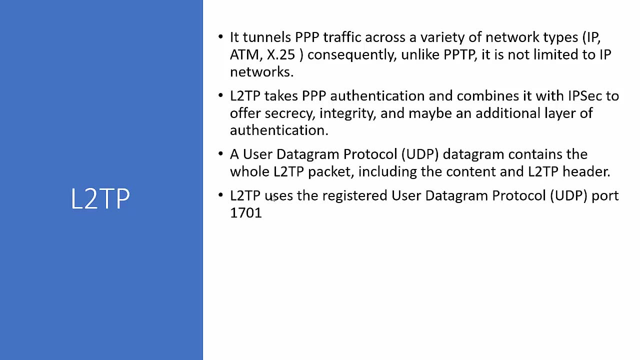 key exchange. they use Diffie-Hellman, so that is a function of IPSec. so I am planning to cover in a separate module about IPSec. so here we talking about L2TP, so L2TP use IPSec, by which it protect the IP packets. so at IPSec, so L2TP, use UDP, so UDP datagram contain the whole L2TP packet which 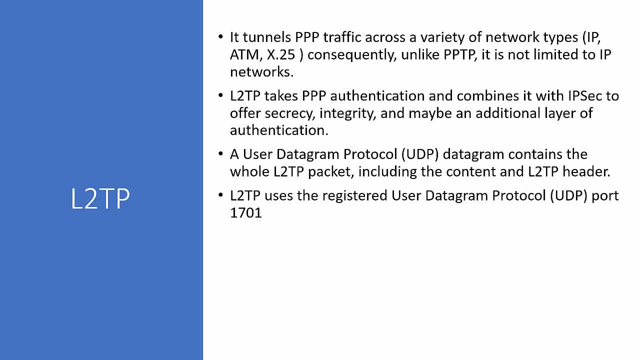 include the content of L2TP header and L2TP use register. UDP port number one: seven zero one. okay, L2TP. we have a two type of message. one is called as a control message and one is called as a data message. when you're talking about the control message, it passes control and data message over. 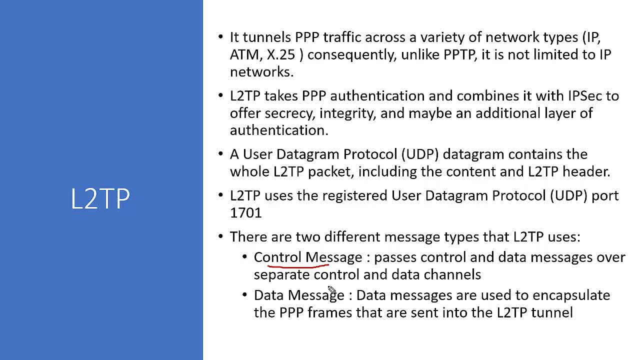 the separate control and data channel. so L2TP passes control and data message over the separate controls and data channel and the inbent control channel pass the sequence controls, connection management, call management, error reporting, session control message and everything okay. and when you're talking about data message, data message used to 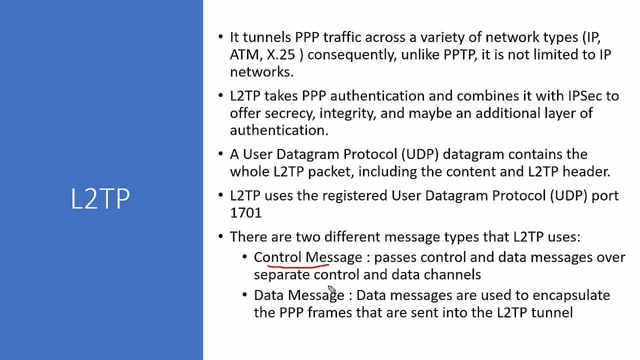 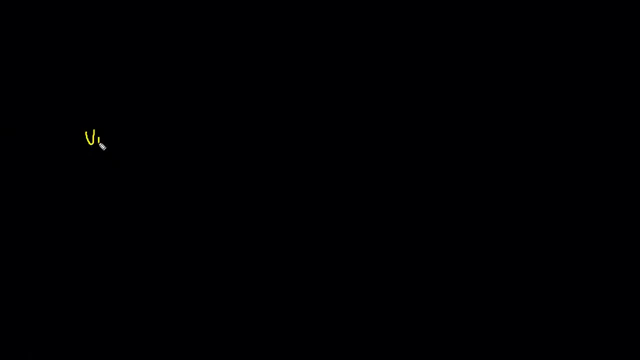 the PPP frame that are sent into the L2TP tunnel. that is basically the two type of message we have. so if you ask me the overall hierarchy of VPN, radius, IPSec, so let me explain that also and then we'll discuss some coffee shots. now, if we take a scenario here, okay, so we have a user one. 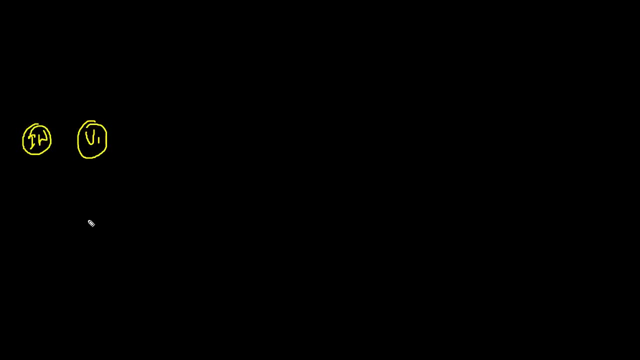 based out in India. we have a user two which is based out in Bangladesh and we have a user three which is based out in Sri Lanka. they are basically connected with the internet. so this is my internet. okay, I'm going to cover radius and techass plus in a separate module, but I thought I will. 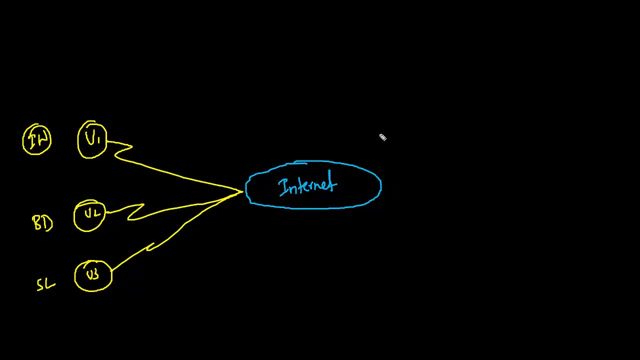 cover a very high level here. okay, as we covering the VPN. now this is my router. let me configure. so this is my router and now what we did. this is basically my enterprise network. this is my enterprise network. okay, now, what I did here is we have a VPN server which listen IP, we have a dial-up server which understand number, and then 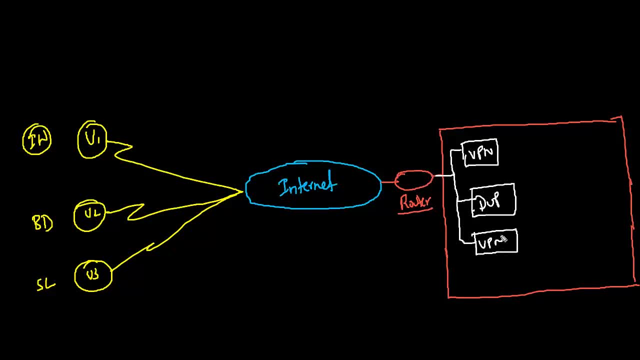 we have another VPN. they all are basically connected with the radius you and radius basically connected with the active directory or certificate authority. you can say ad as a la, also LDAP. so process is now we have a user, so user, basically with the help of internet, do the dial-up, do the IP dialing. 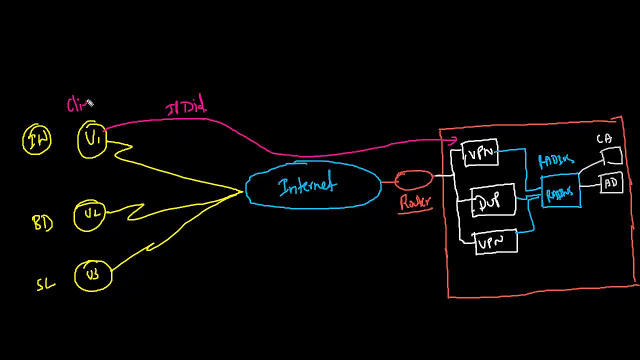 because here the client need to select the connection also, whether you need to go for PPTP or whether you need to go for L2 TP. he select the PPTP, L2 TP from this pointer and by this he send a request to VPN. so this is basically direct. there is a possibility. 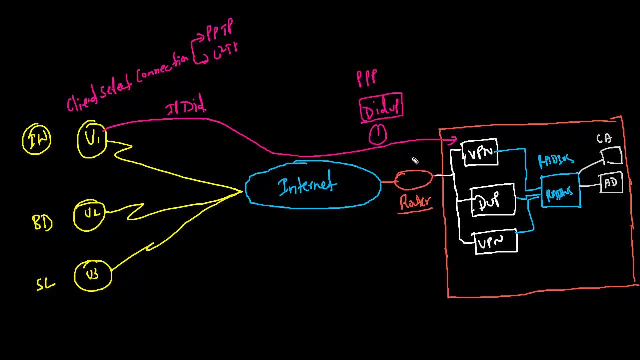 of using a dial-up protocol here which is called ppp, and then, on ppp, we basically have a L2 TP, or or we have a PPTP. then, on ppp, we basically have a L2TP, or or we have a PPTP. 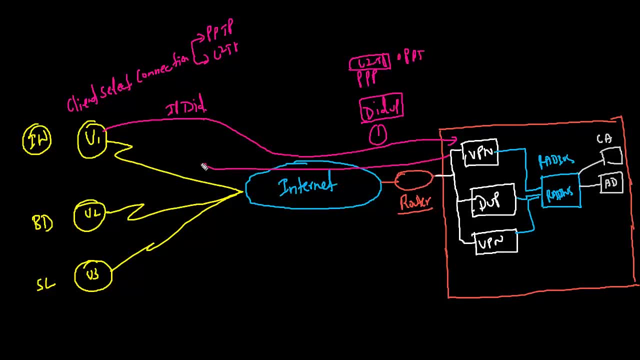 now VPN, basically ask for the username and password. username and password. this time either using CHAP- if using Microsoft, then Microsoft version is called as an MSCHAP- or we have a PAP, which is more concern. then he enter the username password and he send the information to the VPN. now VPN itself. 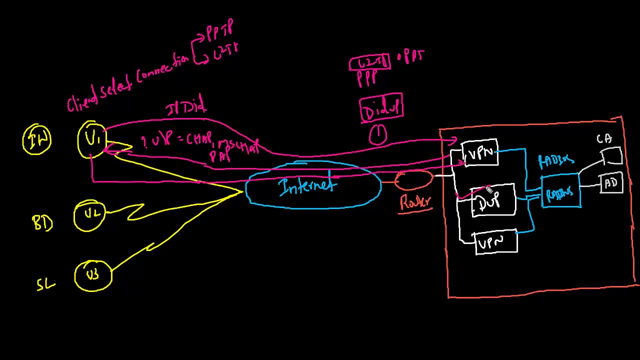 will not do the authentication because we also receiving a request from dial-up. we requesting receive from VPN. we also have an access point here- who receiving a request from multiple users. so what I need here is: I want a centralized identification authentication authorization. I am looking for a. 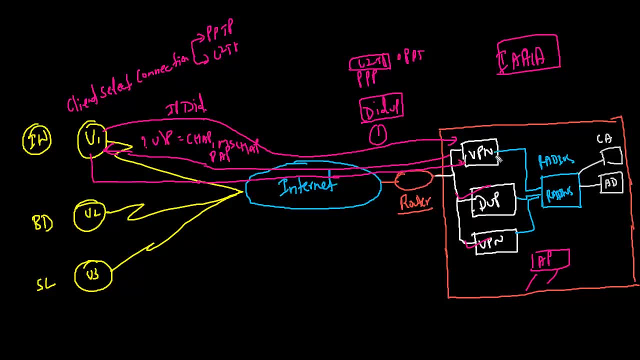 centralized identification authentication authorization. so in that case they will forward the information to radius. radius is act like a intermediate agent to radius. this request is carried by the protocol which is called as a EAP- extensible authentication protocol, because so far the packet does not have an IP. 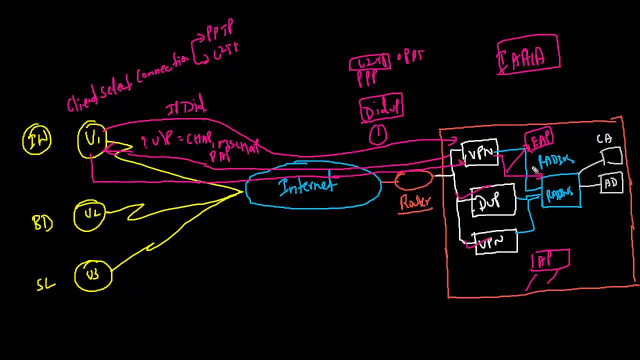 you. so it passed the information to radius. it is carried by the EAP protocol, which work on the layer-2. radius will pass this information to AD. it is just act like a intermediate agent. radius pass this information to AD. AD will authorize and verify and then he authorized the radius. radius will forward this. 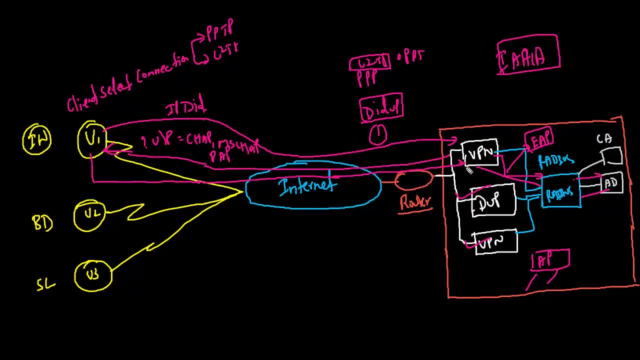 information to VPN, and VPN is basically help us to create a tunnel between these two systems and through this system, it basically transfer the data. so this is is how it works. the radius has a limitation: it work on the UDP protocol and information, which is basically exchanged from radius to AD in a plain text. so in order to secure that, we basically 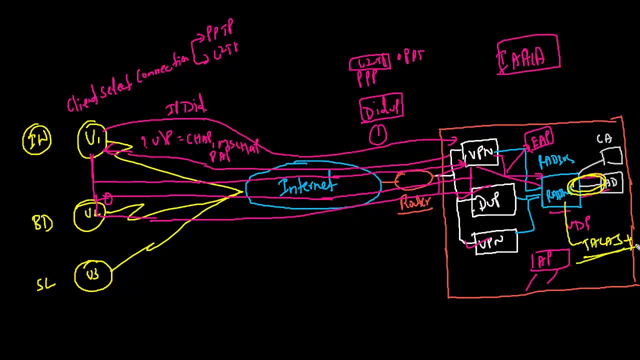 introduce the tech as tech, as plus okay, tech as is basically from a Cisco proprietary. so this is how the overall things works in the systems. I'm planning to cover the radius in a separate module, so if you understand this topic well, let's have a coffee with prep. 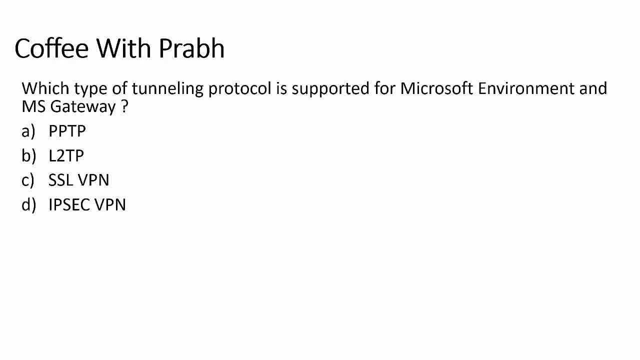 okay. so which type of tunneling protocol is supported for Microsoft environment? the keyword is Microsoft environment or MS gateway. so definitely directly. we remove the L2 TP for the Cisco. SSL VPN is also work, but SSL VPN is a vendor agnostic between. it can work on the. 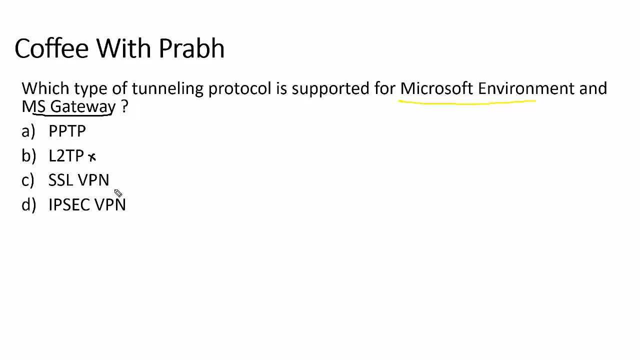 browser base and all that. and from exam point of view, remember that SSL VPN does not require any kind of a configuration: open the browser and connect. so when we looking from the point of view of a least configuration, less tedious task and all that, we can go for SSL VPN. 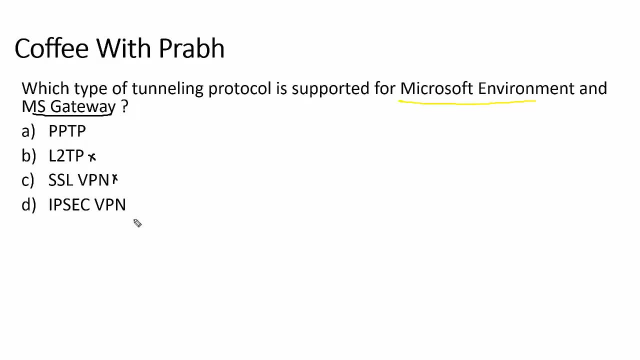 IPSec VPN. there's nothing called as IPSec VPN. VPN is work with L2, TP and all that. so that is removed. so only option is basically left is a PPTP. that's where the answer is a for alpha. let's move to the next coffee shot. what is the primary limitation with PPTP? PPTP support layer 3. that is a advantage. that is not a limitation. PPTP doesn't support the layer 2 WAN protocols. that is true. PPTP do support layer 2 WAN protocol. it is a wrong statement itself. PPTP send the data in plain text, which is a wrong statement. so only option which is very close is BB. PPTP does not. 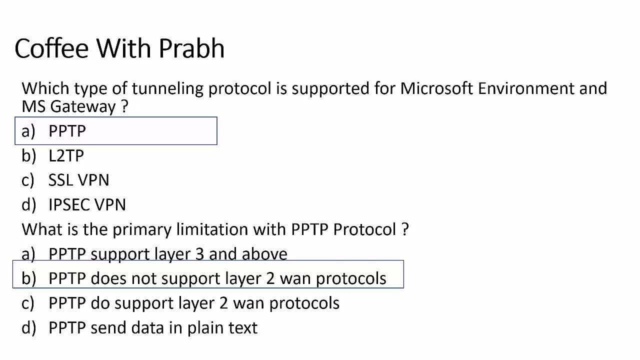 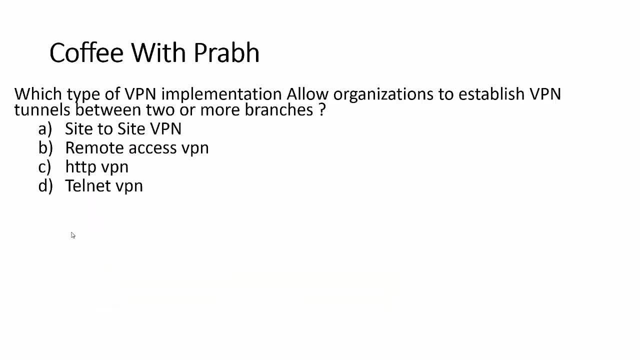 support layer 2 WAN protocol. that is why we introduce the L2 TP PPTP support from a layer 3 onwards for the Microsoft understanding. okay, so which type of VPN implementation allow all organization to establish VPN Tunnel between two or more branches? option is site-to-site VPN option. 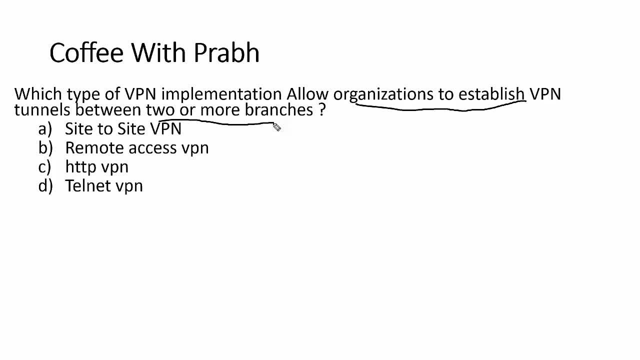 be remote access. VPN. option C, HTTP and option detail net C and D is not there, so we left with a and B the keyword talking about here two more branches. so answer is basically: site to site VPN. which VPN type inherit PPP authentication integrate with the IPSec to provide confidentiality? 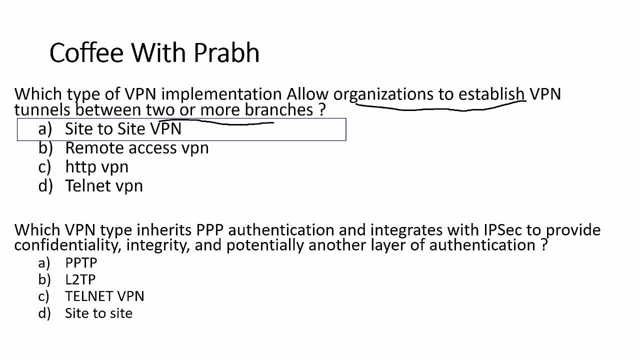 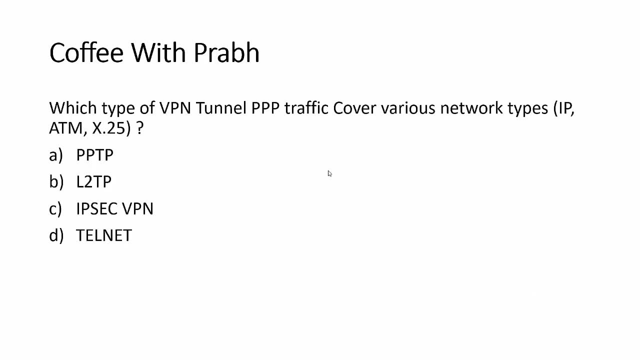 integrity, potentially another authentication. we know that the answer is basically L2 TP, because PPTP has the limitations. so let's move to the next part. which type of VPN tunnel PV traffic cover various network type: ATM, IP and x.25? so answer: PPTP doesn't support. 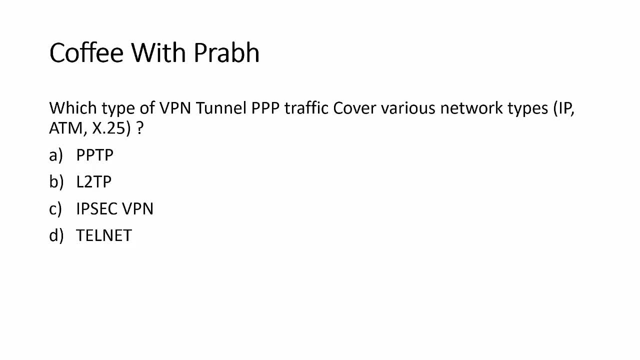 because these are work on the layer 2. there's nothing called as IP, say VPN. telnet is for remote administration, so only option is basically left is L2 TP. so if you find this video useful, do share in a network and let me know what are the new videos you want me to create. if you new to my channel, do subscribe to. 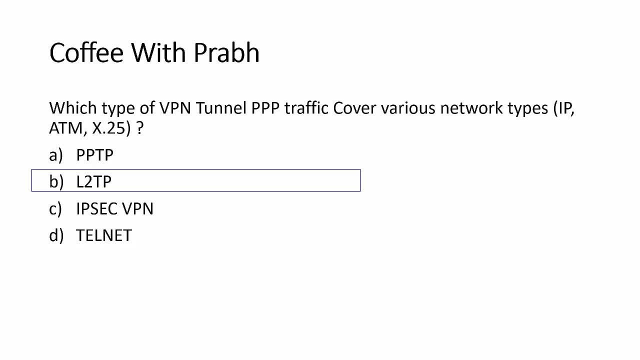 my youtube channel. I am coming with more videos like that, with questions, mapping, so by which we can able to have a visibility about the topics. and do subscribe to my youtube channel. okay, guys, you. and before we wrap up small assignment, do let me know some example of layer 2. 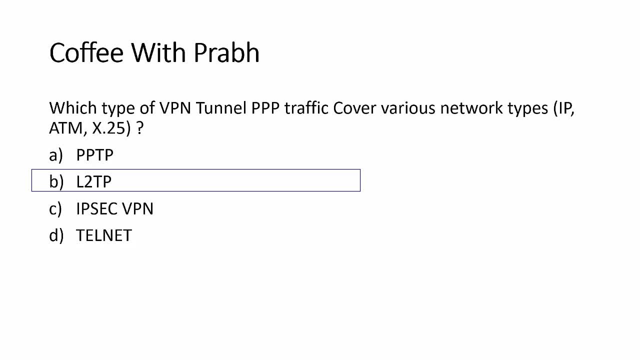 communication protocol and IPSec limitation in the comment box. thank you,